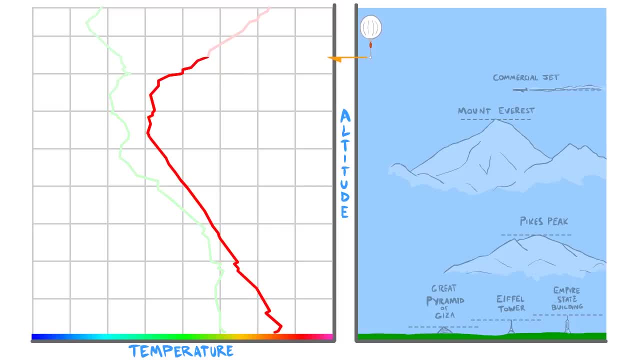 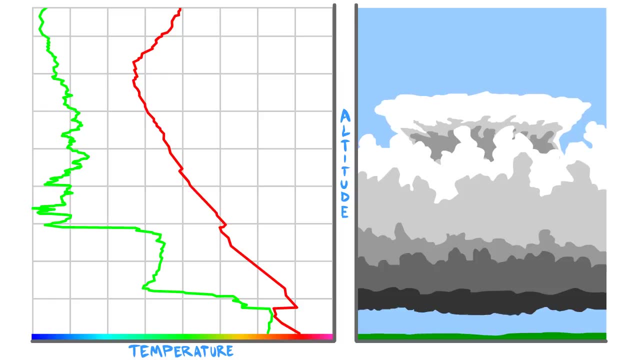 see in this graph. It's interesting to note, however, that really high up it begins to get warmer again once you enter the stratosphere. This particular sounding tells scientists to watch out for severe weather, including tornadoes. Here is another example that may. 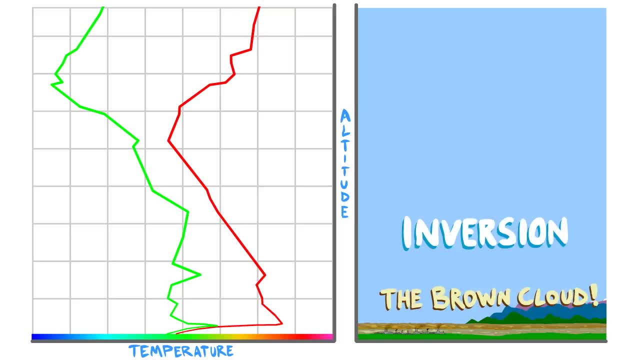 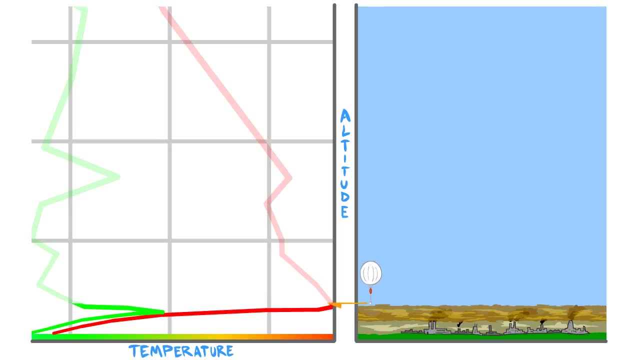 in Colorado know as the brown cloud called an inversion. Here you can see at the beginning of the launch. near the surface it's actually getting warmer as it rises. Then we can see where it immediately gets colder. This is where the colder layer of smog is trapped. 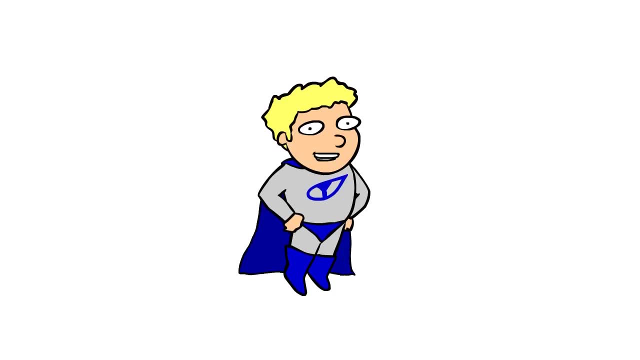 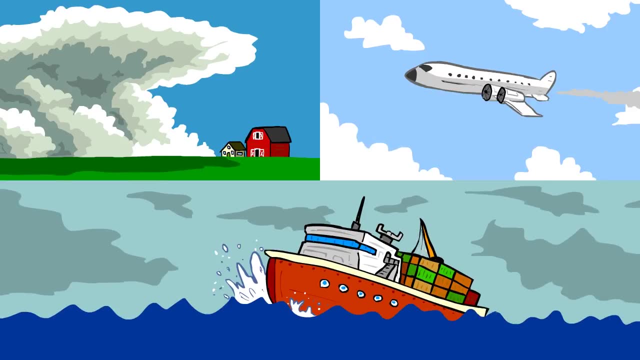 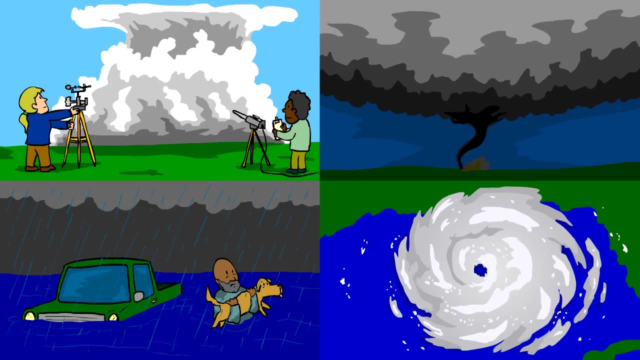 below the warmer air above. But that's not all the data are used for. We use it for local severe storm prediction, aviation and marine forecasts, Field programs to study specific atmospheric phenomena like severe thunderstorms, tornadoes, monsoons and hurricanes. It's used for ground truthing, where observations 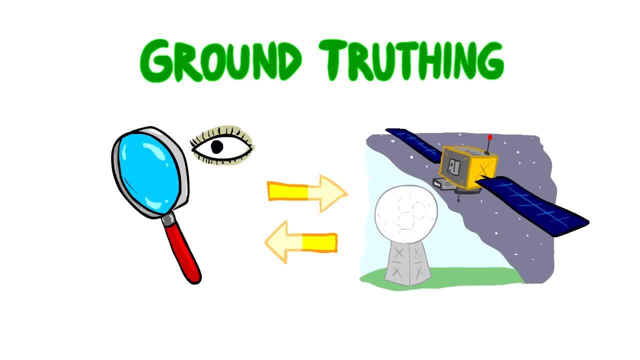 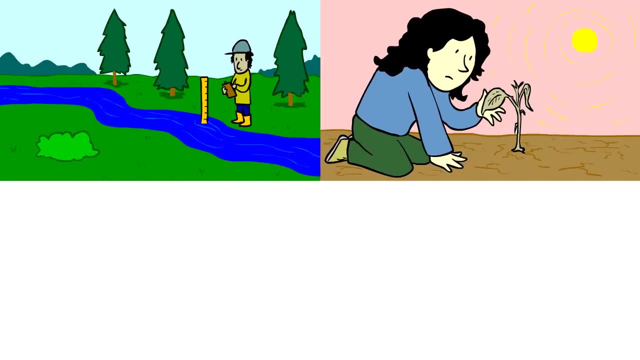 are compared to check the accuracy of radar and satellite data, And the data are also plugged into many different kinds of useful modeling tools which can help predict river and stream levels, the onset of drought, pollution and air quality, and even the spread of certain 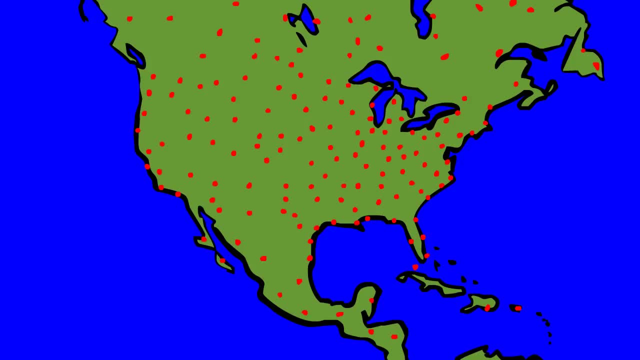 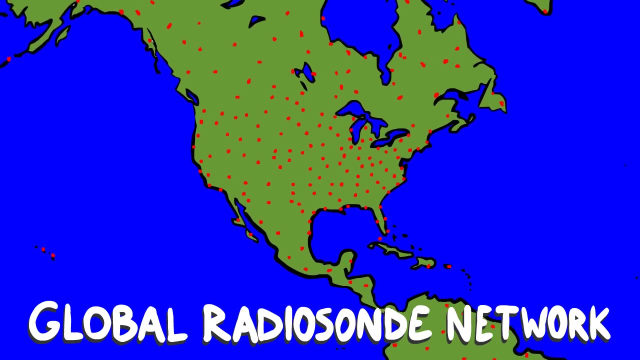 mosquito-borne diseases. 92 sites in the US launch weather balloons simultaneously twice a day. This is part of the Global Radiosonde Network With over 900 sites that provide the observations to accurately describe our current weather and make accurate future forecasts.